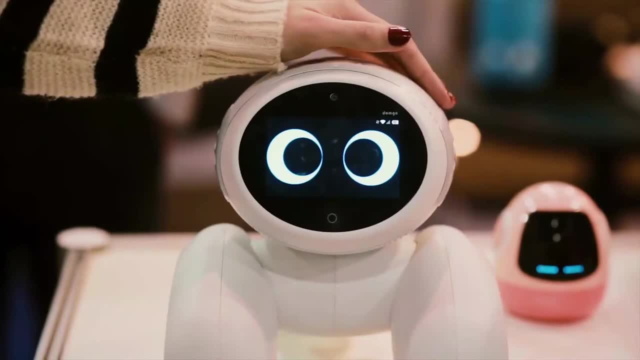 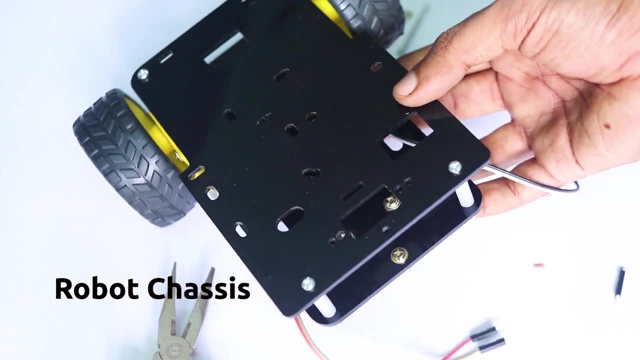 projects on your own. make sure you subscribe to our channel. So let's get started About the robot chassis. this is something I bought online from Amazon. As you can see, there are two wheels connected on either side of this robot chassis. These two wheels are 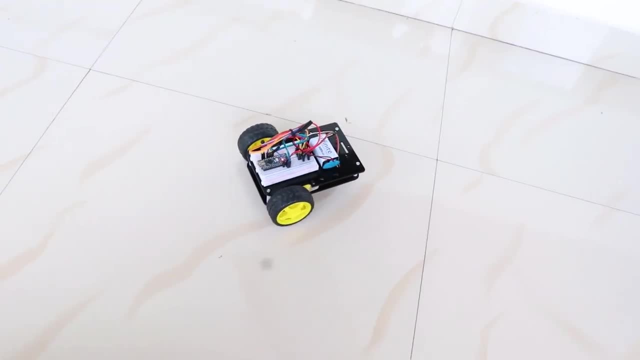 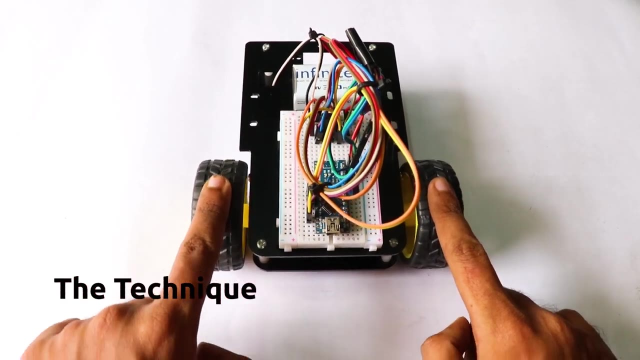 connected to two DC motors. The entire movement of the robot is controlled by the direction of rotation of these DC motors. That is, when both these DC motors rotate clockwise, the entire robot goes forward. Likewise, when both these DC motors rotate counterclockwise. 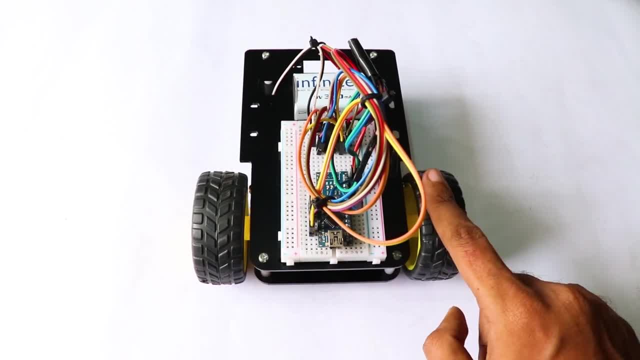 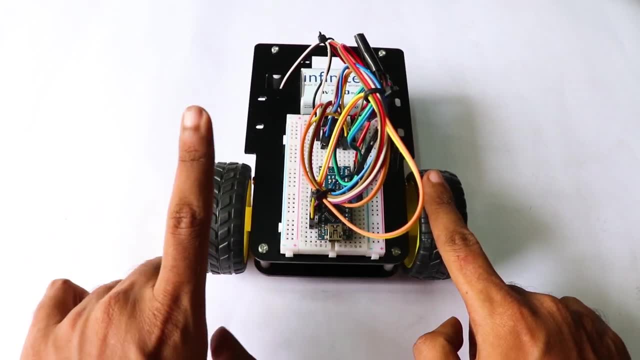 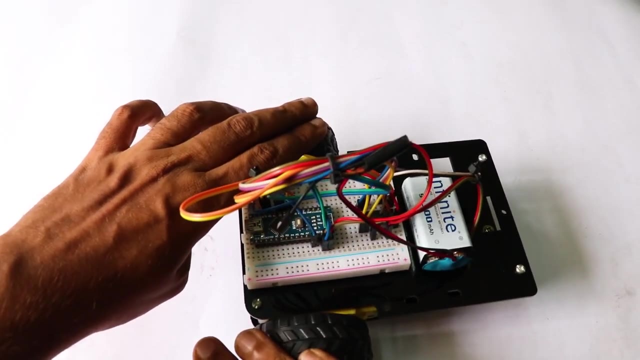 the robot goes backward. Now, when the right motor stops and the left motor rotates clockwise, the robot turns right, Like that. when the left motor stops and the right motor rotates clockwise, the robot turns left. That's cool, right, When both motors rotate in opposite directions, one clockwise. 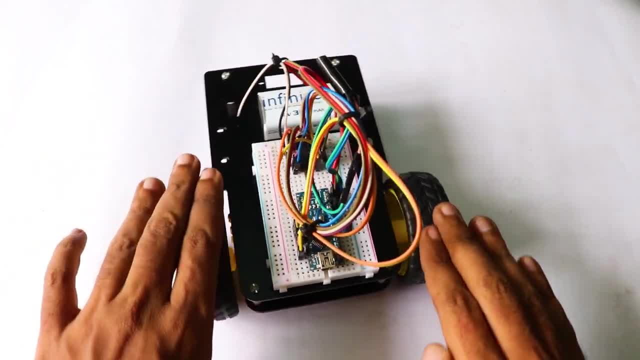 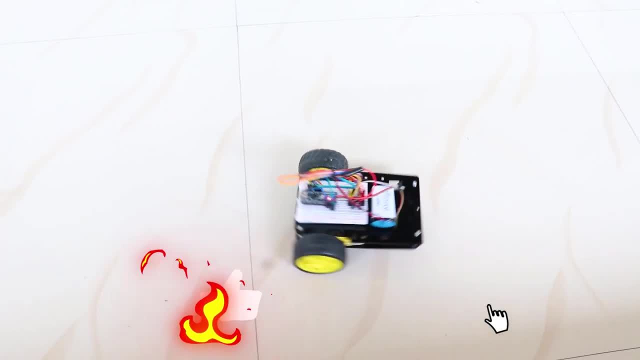 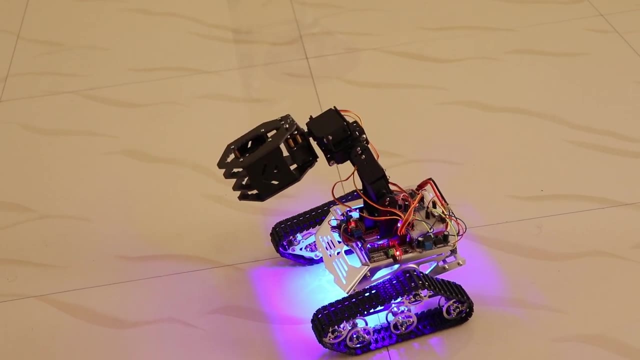 and the other. anticlockwise, the robot turns from that position itself. Simple as that. And that's how you control the movement and direction of a simple robot using two DC motors. Thanks for watching. Now, that was easy, right? If you have any doubts regarding any DIY electronics projects, 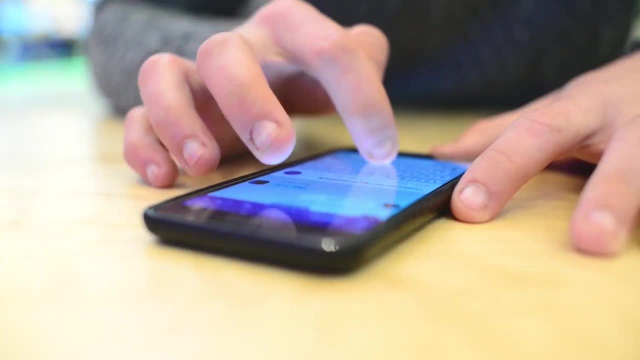 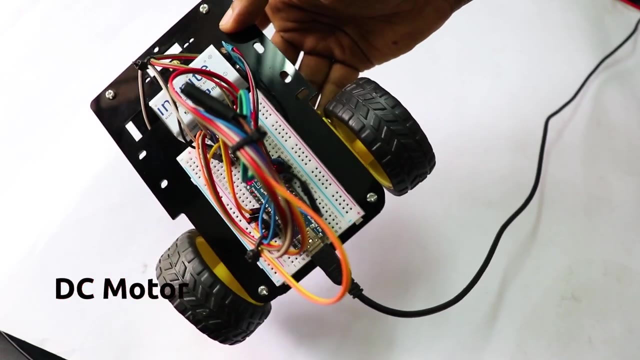 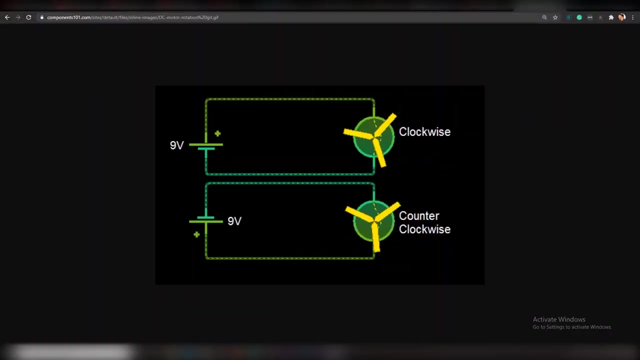 just shoot it out in the comment box below and make sure you use our WhatsApp group to clear all your doubts and show off your projects. The next task is to control the direction and rotation of the DC motors, to control the robot the way we want. One specialty of the DC motor is that it can rotate in both directions. 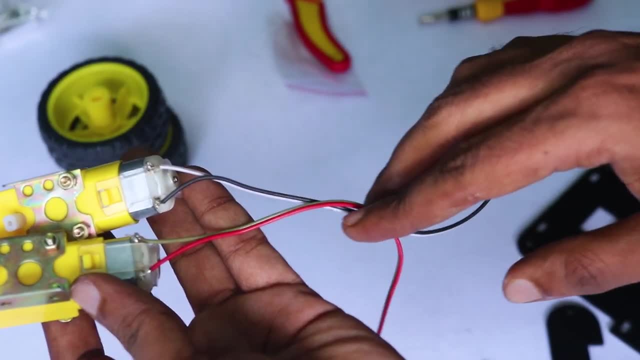 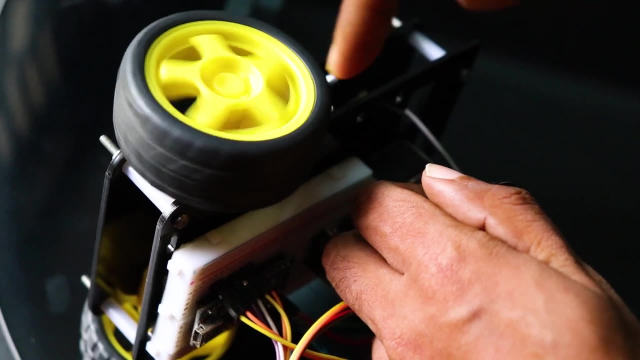 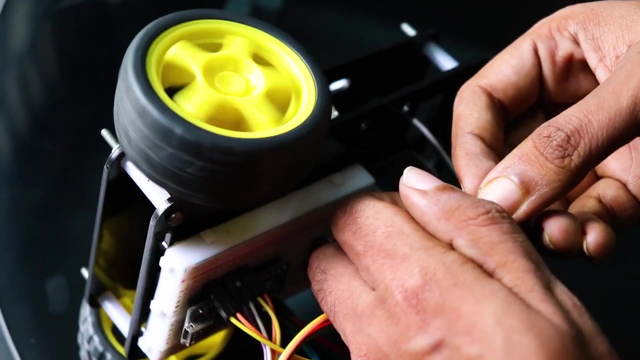 clockwise and anticlockwise. The DC motor has two terminals, terminal A and terminal B. If the motor rotates clockwise when terminal A is connected to positive terminal and terminal B to negative terminal, it will rotate anticlockwise when this polarity is reversed, That is, when terminal B is connected. 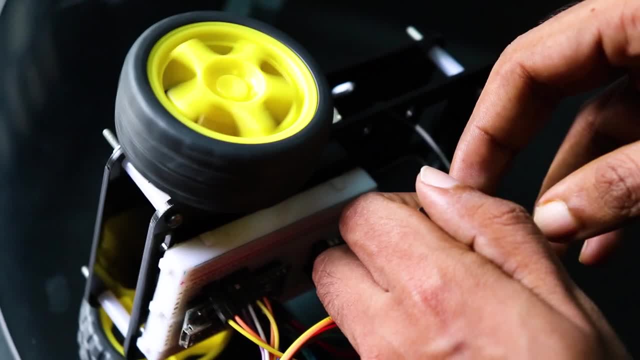 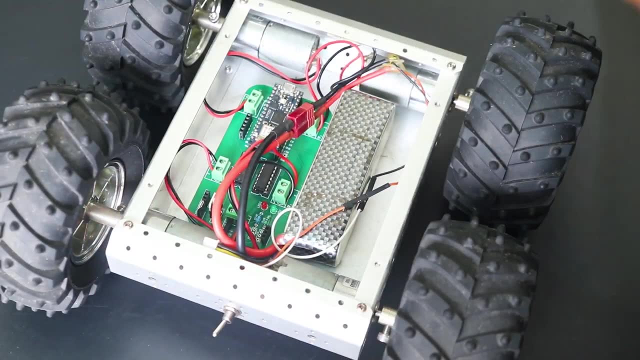 to positive and terminal A is connected to negative. All you have to do is reverse the polarity. But in the case of a robot, it's not always possible to disconnect and connect DC motors to chase the polarity and control the direction. So what do we do in that situation? 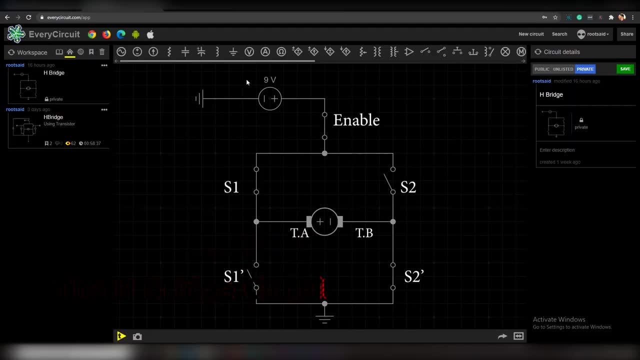 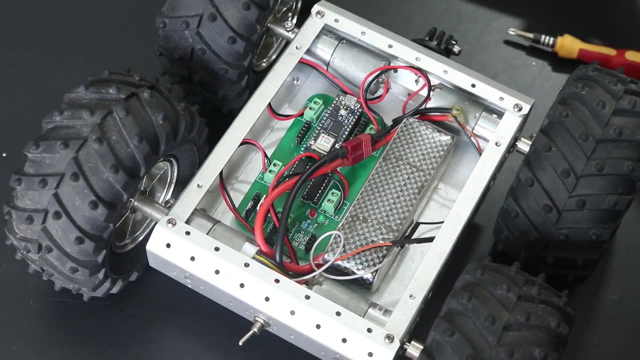 We'll see. in the next video, We will use a simple circuit known as H-bridge. Ever heard of it before Now? this circuit is something that we knowingly or unknowingly use in almost all of our robotics projects. Don't worry, guys, if you don't know it, I'll be explaining in such a way that it'll be. 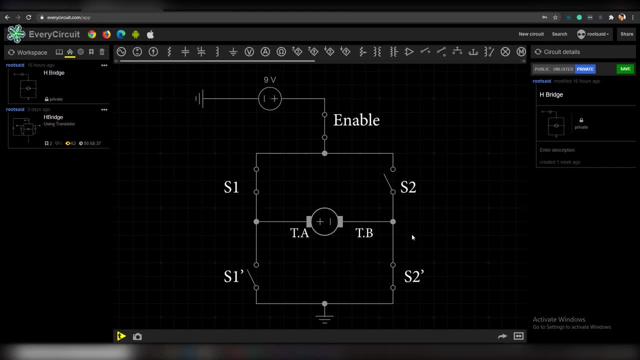 very easy for you to understand. Now. this is a simple H-bridge circuit. There are mainly four switches: S1-S1- and S2-S2-. Now, if you take a closer look, you will see another switch right here. Its name is never. 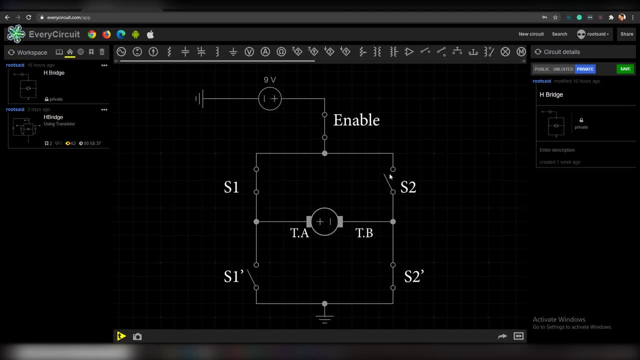 forget the cable switch In this circuit. S1 and S2 will be the two switches that will be under our control. S2- will be the complement of S2 and S1- will be the complement of S1.. That means when S1 is 0, S1- will be 1 and when S1 is 1, S1- will be 0. The same goes. 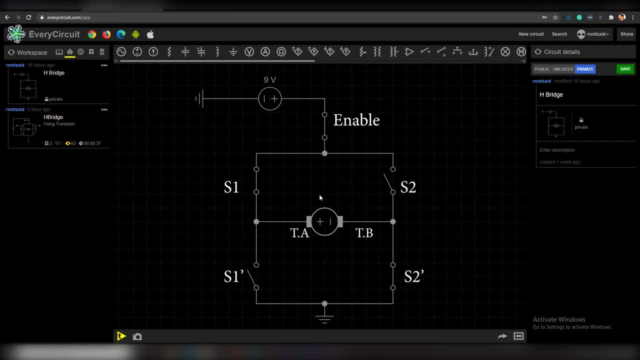 with S2 and S2-, And here you can see a DC motor connected in between, And the whole circuit is powered by a 9V battery. Now let's close S1 and open S2. And let's see what happens When S1 is closed, S1- will. 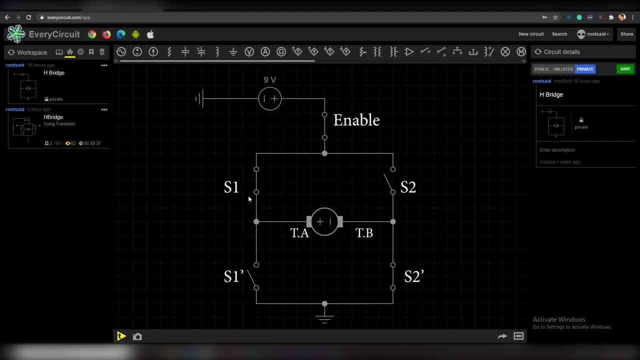 be open. Why? Because S1- is the exact opposite of S1. Similarly, when S2 is open, S2- will be closed. At this time, this is how the circuit looks like. The current flows from positive terminal of the battery through enable switch, switch S1, terminal A of DC motor, terminal B of 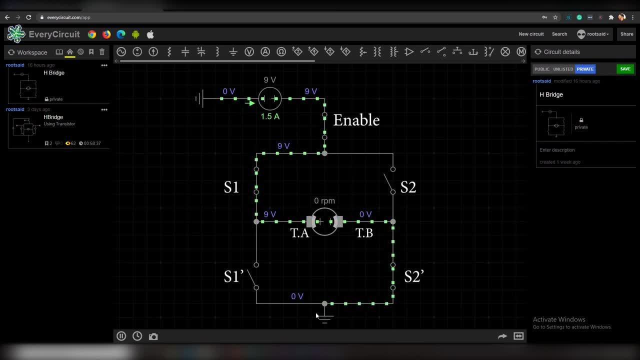 DC motor to S2- and to the negative terminal of the battery. Now, if we take a closer look, we can see that terminal A of DC motor is connected to positive terminal of the battery. at the same time, terminal B is connected to negative terminal of the battery. Now, 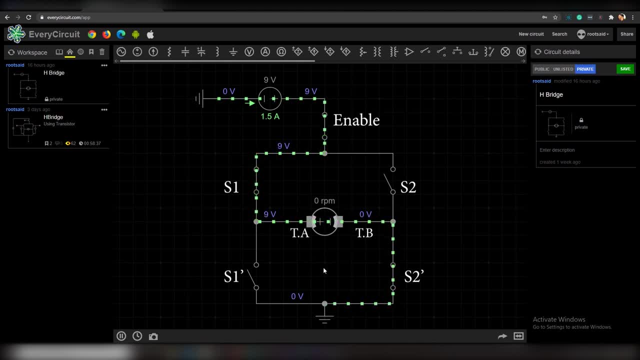 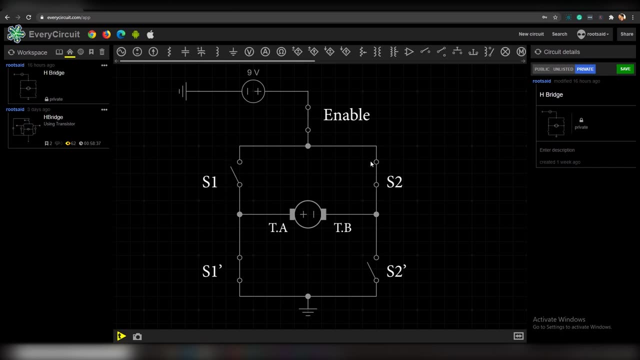 the motor will be rotating in clockwise direction. That was easy. right Now, let's open switch S1 and close switch S2.. And see what happens: When S1 is open, S1- will be closed, and when S2 is closed, S1- will be closed. 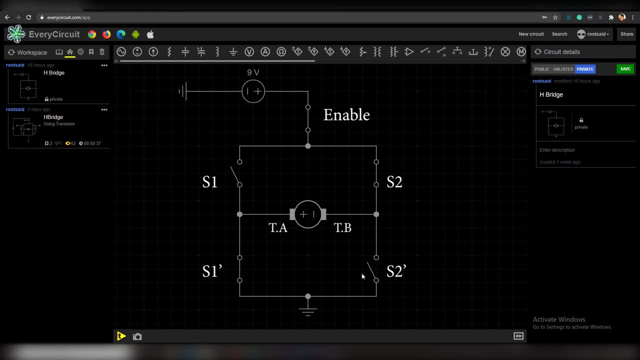 S2- will be open, Exactly the opposite of previous case. This is how the current flows This time. current flows from positive terminal of the battery through enable switch, through S2, through DC motor, from terminal B to terminal A, through S1- to negative terminal of the. 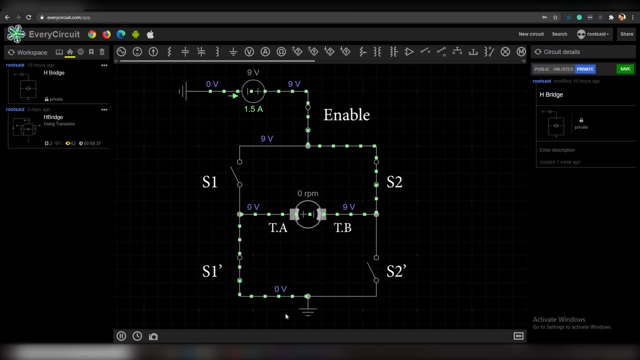 battery. You got the point right. This time everything is inverted. Now terminal B of DC motor is connected to positive terminal of the battery and terminal A of DC motor is connected to negative terminal of the battery. This time DC motor rotates in anti-clockwise. 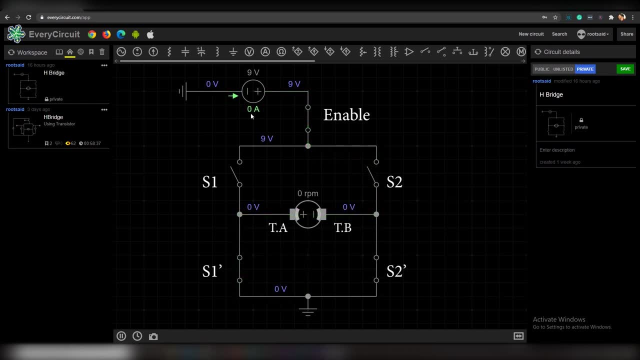 direction. Exactly the opposite as before. Now, when S1 and S2 are both open, S1- and S2- will be both closed, But the circuit is open. That means there is no way for the current to travel from positive terminal of the battery to negative terminal of the battery. So the 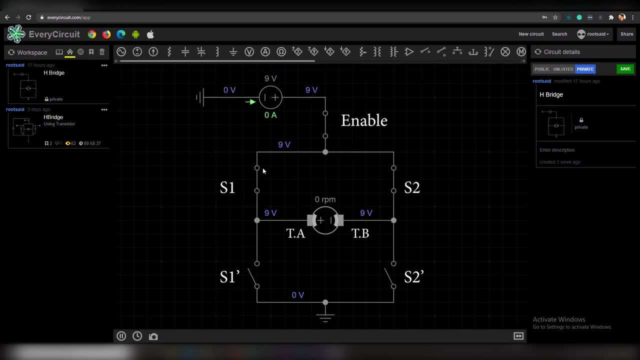 motor will not be rotating when S1 and S2 are closed. When S1 and S2 are closed, S1 dash and S2 dash will be opened. This time also, circuit will be opened and the motor won't be rotating. This is how we control. 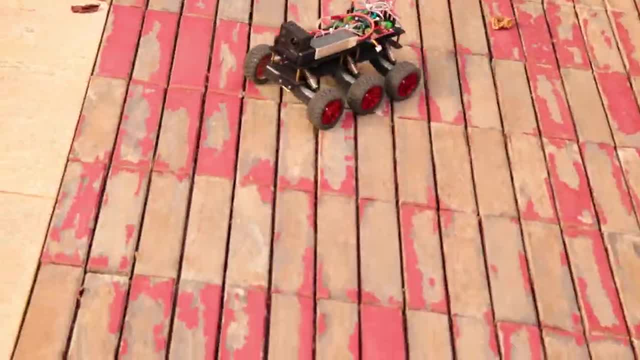 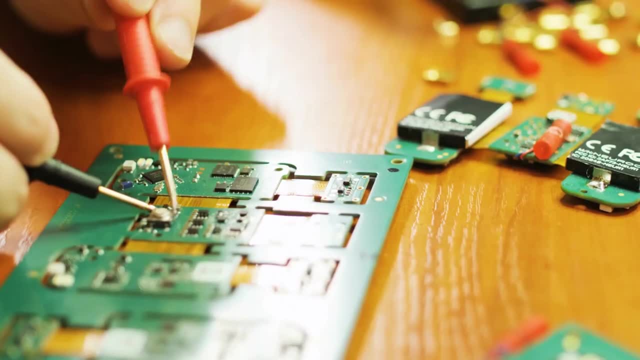 the direction of DC motor using Hedge Bridge Motor Driver. I hope you understand everything easily using this visualization. If you did understand, don't forget to hit the like button Now, instead of S1 and S2, you can use any switching element like a push button switch. 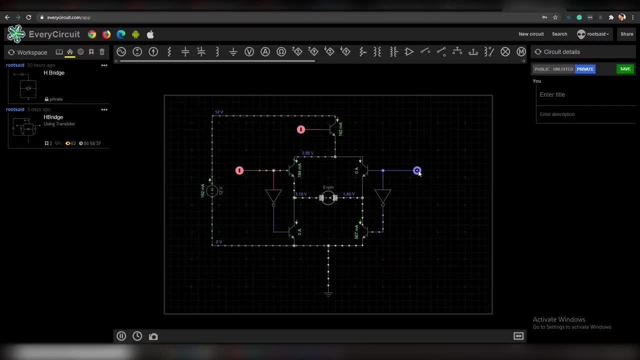 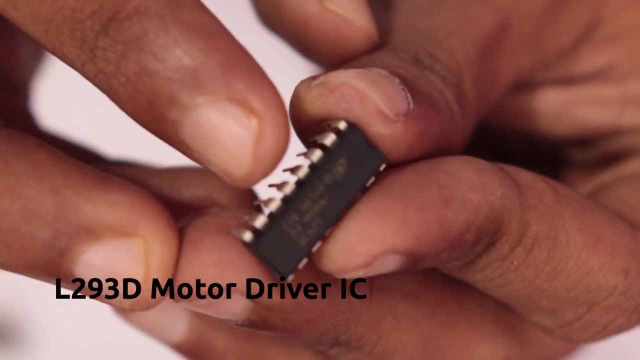 BJT or MOSFETs. Anything would do By doing so. we can open and close these switches by providing 0V over 5V using Arduino microcontrollers. This is exactly what L293D Motor Driver IC consists of. It has two independent H-Bridge circuits which will 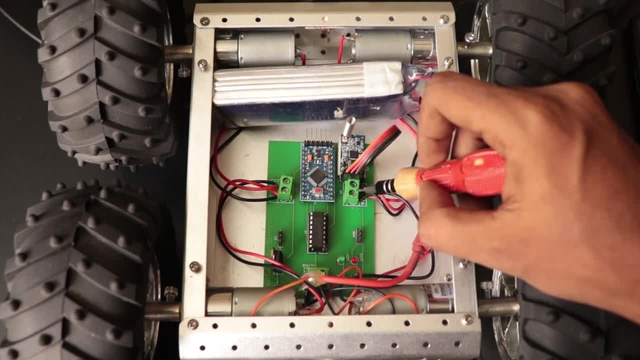 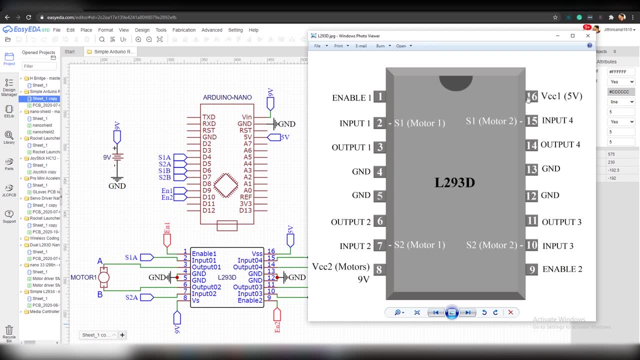 enable us to control two sets of DC motors independently without any hassle. Now let's take a look at the pinup. Here we can see that there are two power sources: VCC1 and VCC2.. VCC1 in pin number 16 and VCC2 in pin number 8.. 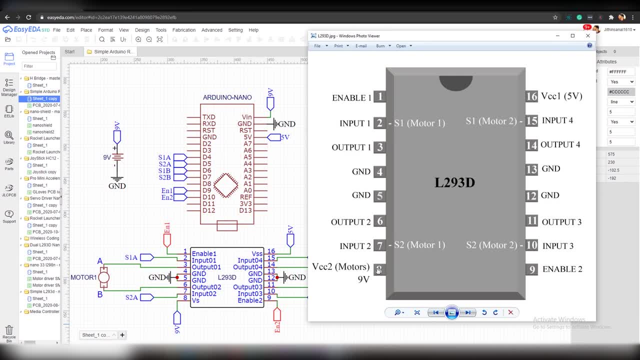 Why do we need two voltage sources? We will be connecting the voltage source which is required to drive the motors in pin number 8.. In our case, we will be connecting 9V battery to pin number 8.. And we will be connecting 5V to pin number 16 or VCC1. 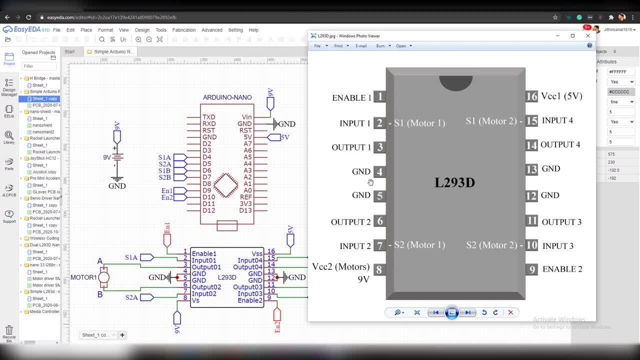 which will be used for internal logical operations of this L293D Motor Driver IC. Then we have four ground pins which are internally connected. Then there are two sets of inputs and outputs On either side of the IC. we will be controlling motor 1 using the left side pins and we will be 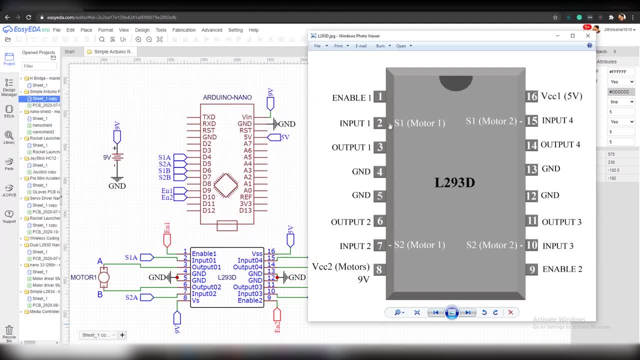 controlling motor 2 using the right side pins. Pin 2 and 7 are the S1 and S2 switches that we saw earlier in the H-Bridge circuit. We will be able to control the direction of the DC motor by providing logic 0 and logic 1 signals at pin 2 and pin 7.. That is input 1 and input 2 connected. 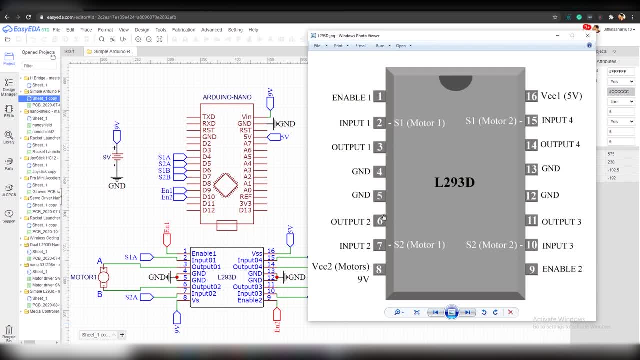 to S1 and S2.. Then we will be connecting our DC motor's terminal to output 1 and output 2.. Terminal A to output 1 and terminal B to output 2.. Then we have one enable pin for each H-Bridge circuit. 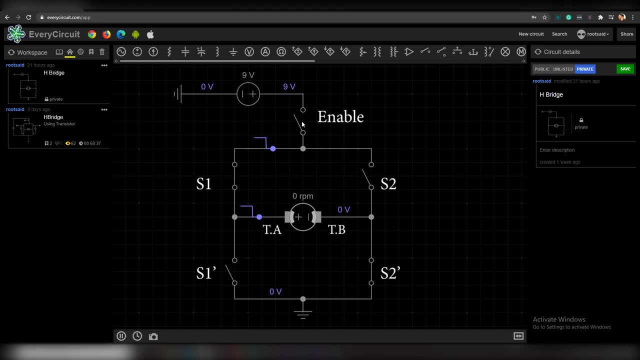 Now this is the enable pin of H-Bridge circuit. The H-Bridge circuit will work if, and only if, the enable switch is closed, It can be considered as a master switch of this whole circuit. That means if enable pin is connected to 0 and even if we are providing correct signals to S1. 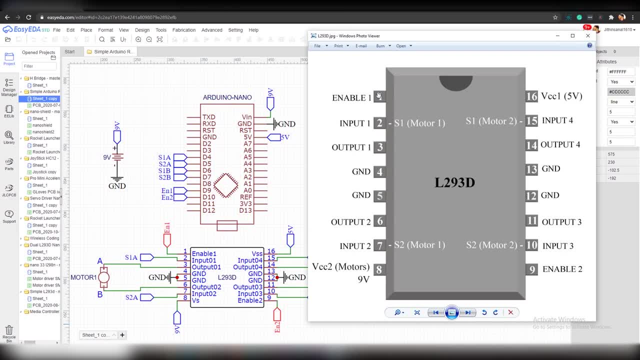 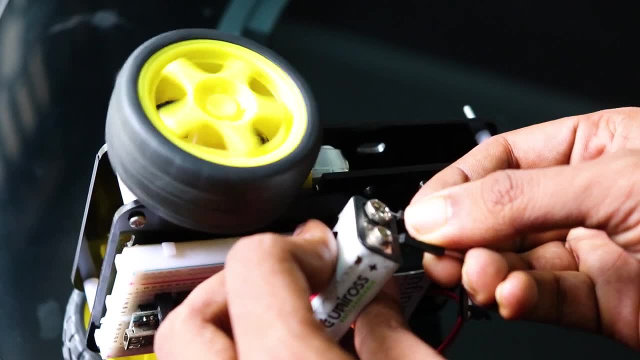 and S2, the motor won't be rotating. One important application of this pin is we can control the direction of the DC motor by providing PWM signals to this pin. PWM signals means Pulse Width Modulated signals. I will explain that in another video. We won't be using that in this robot. This. 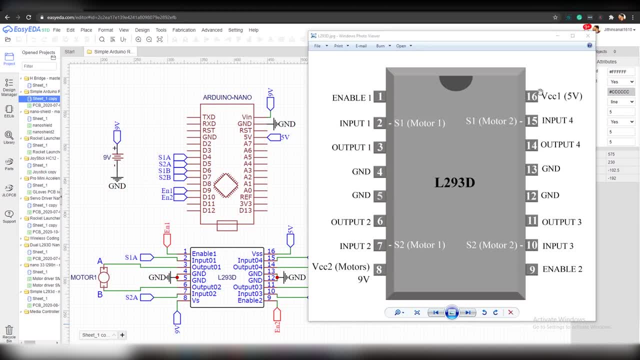 is exactly how we control the direction of the DC motor connected to the other side. Almost everything is ready. just one question remains: How are we going to control switches S1, S2 and enable? That's where our Deno comes to play. Now we are going to connect S1 and S2 of. 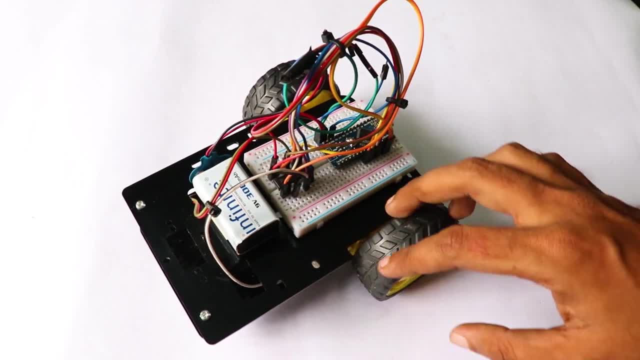 motor 1 and S1 and S2 of motor 2.. Now we are going to connect S1 and S2 of motor 1 and S1 and S2 of motor 2 to our Deno. We will also be connecting both enable pins to our Deno board Once we have. 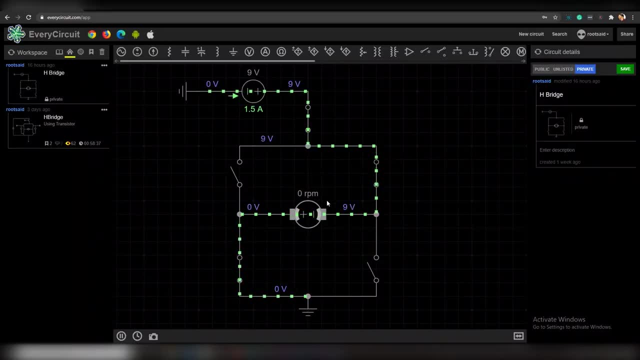 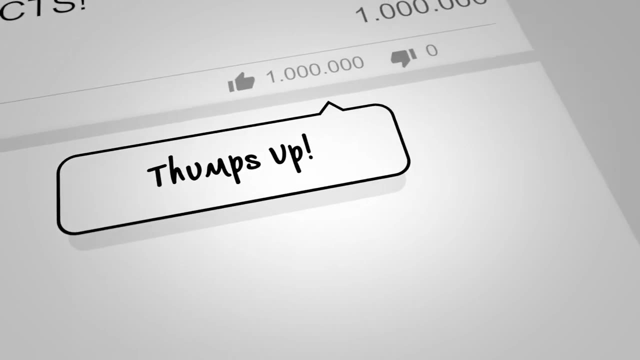 connected them. we will be controlling all the six switches by using our Deno. Let me give you a summary of the circuit. Guys, before going further, if you find this video useful, consider supporting our channel by giving this video a like and subscribe to our channel by clicking the. 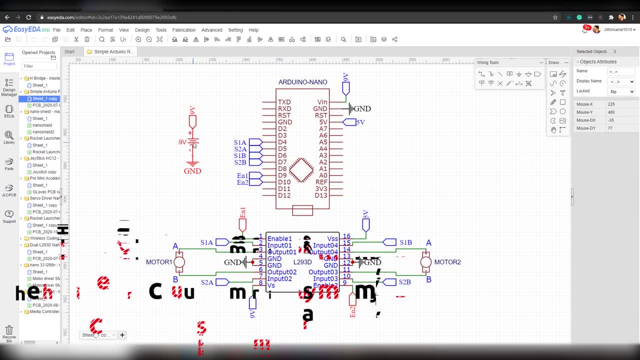 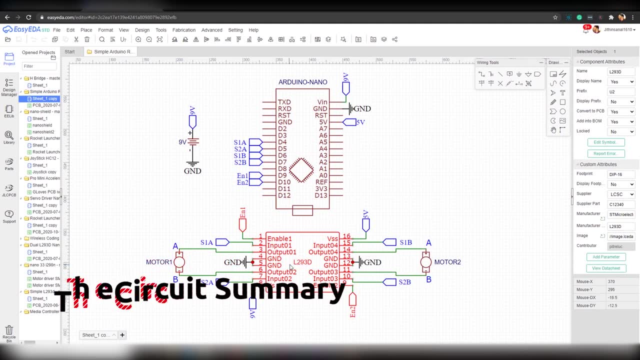 subscribe button below. I would really really appreciate it. Here we have a 9V battery, an Arduino Nano and an L2930.. As you can see here, two output pair of L2930 motor driver IC is connected to two DC motors. 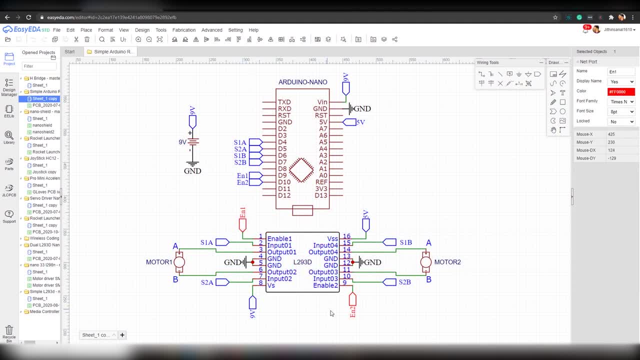 Then we have two enable pins, EN1 and EN2.. They will be turning on and turning off. the motors EN1 and EN2 are connected to the digital pins D9 and D10 of Arduino. Now inputs of motor 1,. 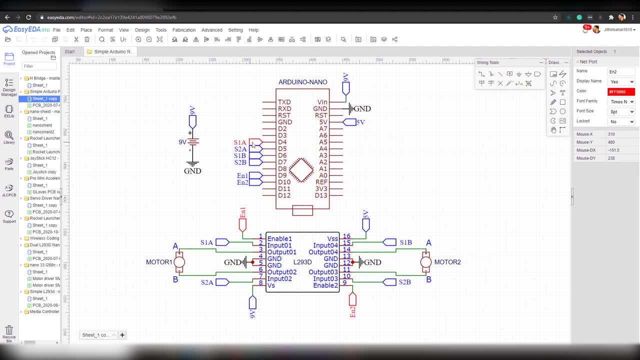 that is S1A and S2A, are connected to D4 and D5 of Arduino. Similarly, on the other side of the IC, the inputs to motor 2, that is, S1B and S2B- are connected to digital pins D6 and D7 of Arduino. 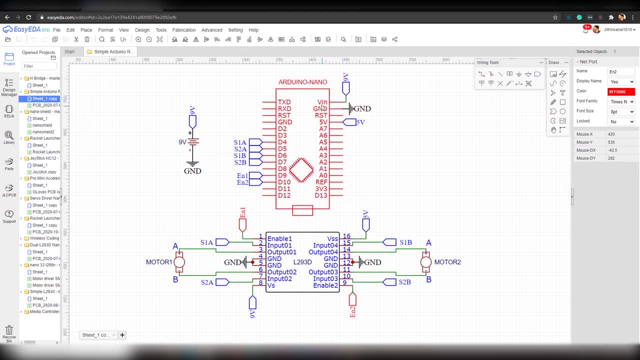 Now the positive terminal of 9V battery is connected to VIN pin of Arduino. This 9V is converted to 5V using a voltage regulator in Arduino Nano and will be available with a 5V pin. This regulated 5V is connected to pin number 16. 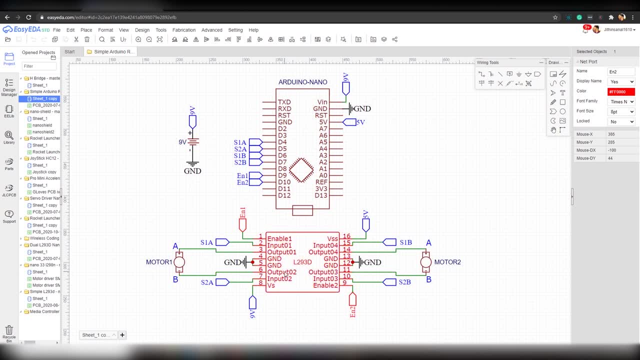 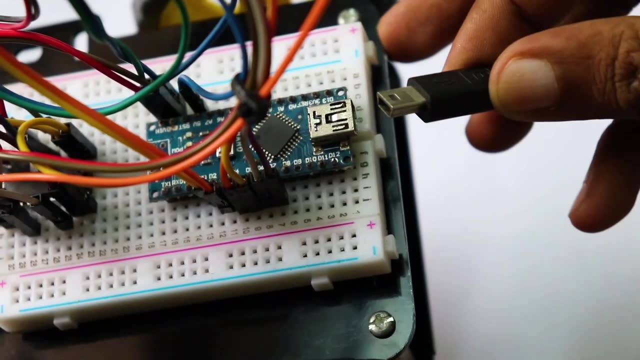 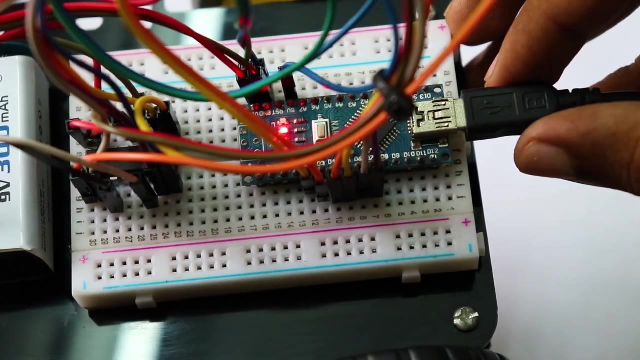 of L2930 motor driver IC. The IC will be functioning using this voltage supply. We will be connecting 9V directly to pin number 8 of L2930 motor driver IC, which will be used for driving motors. Now all you have to do is code Arduino to change the value of enable 1, enable 2, S1A. 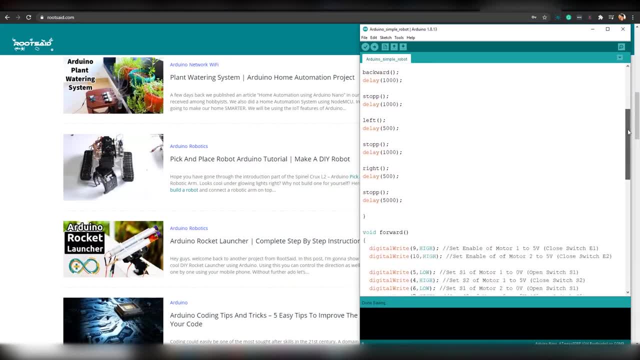 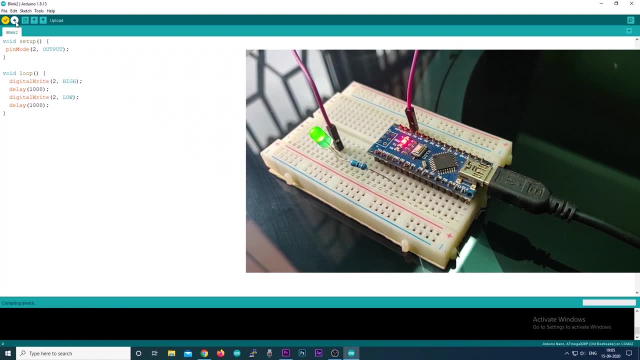 S2A, S1B, S2B to drive the motors. And here is the code to our simple robot. If you are not familiar with Arduino or Arduino coding and you want to start from scratch, make sure you watch our previous video where we explained everything about Arduino. you want to know. 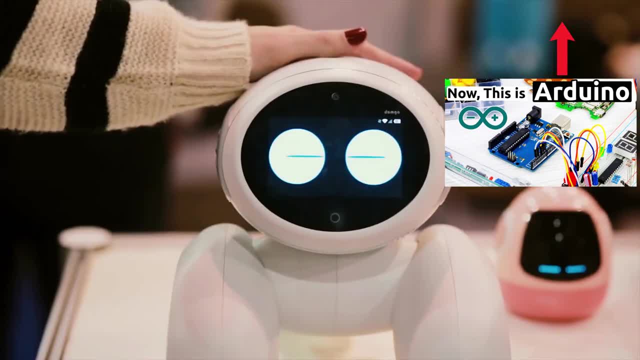 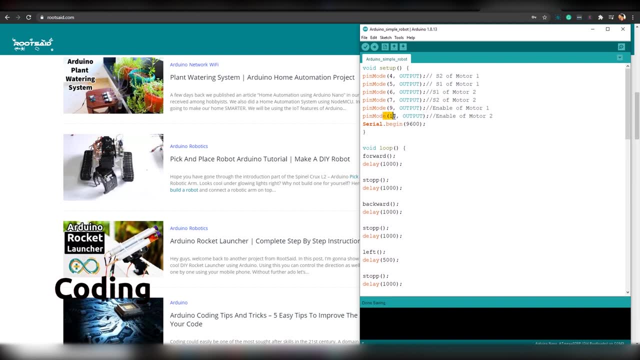 in a fun and easy way. make sure you watch that video, as it's gonna be really useful for you guys. the link will be in the description in the setup function. pin number four, five, six, seven and nine ten: the six inputs to l293d motor driver ic as set as output pins- another thing we are doing in the setup function: 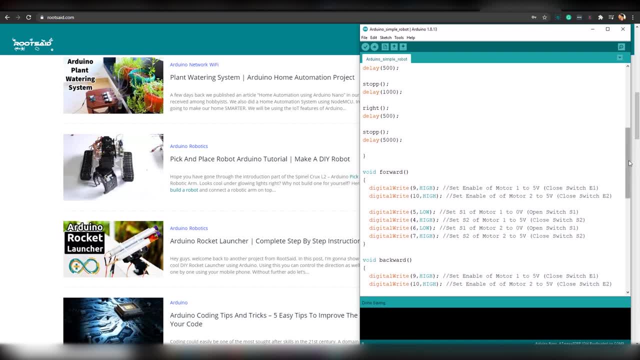 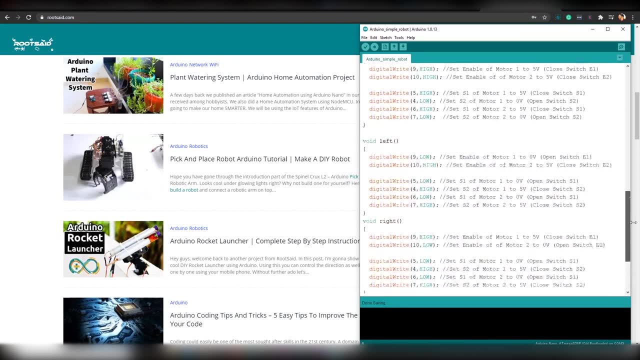 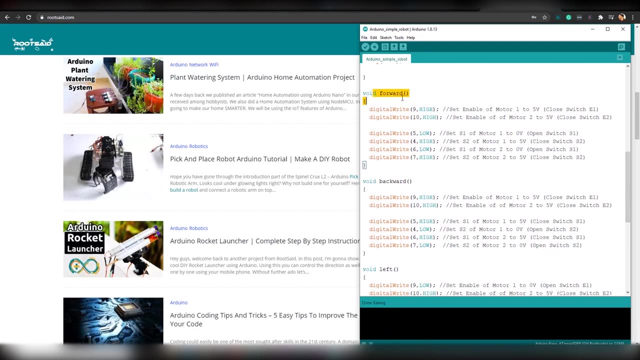 is, we are initializing serial communication. below that you can see five functions: forward, backward, left, right and stop. these are the functions that we'll be using to set the value of switches in l293d motor driver ic. that's how we'll be controlling the motors. now let's check the. 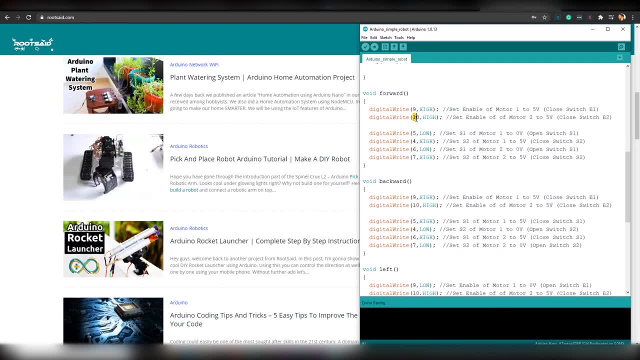 first function forward. here we are setting the value of enable 1 and enable 2, that is, d9 and d10, as true. that means both s bridge will be on. then we are setting s1 off and s2 on for both s bridges. at that time both motor will be rotating in clockwise direction.